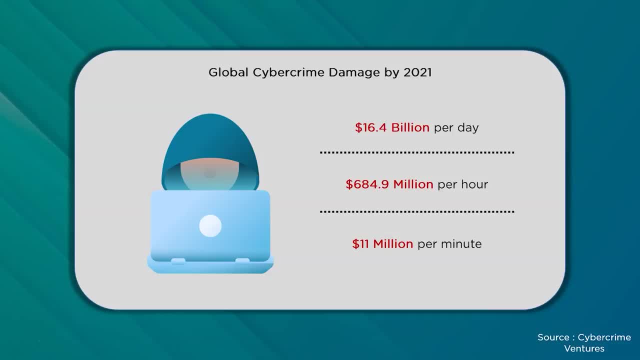 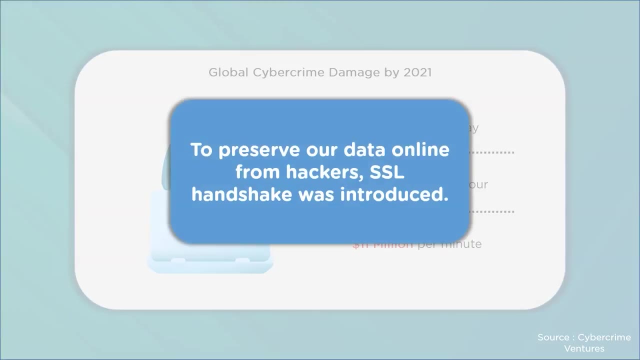 years, The average data breach crossed at $6.84 million, as per 2020 records. Opportunities breed innovation, and this has been observed in the cybersecurity domain as well. To safeguard against such threats, the SSL protocol was developed. Hey everyone, this is Bhavab from Simply Learn, and welcome to this video on the SSL handshake. 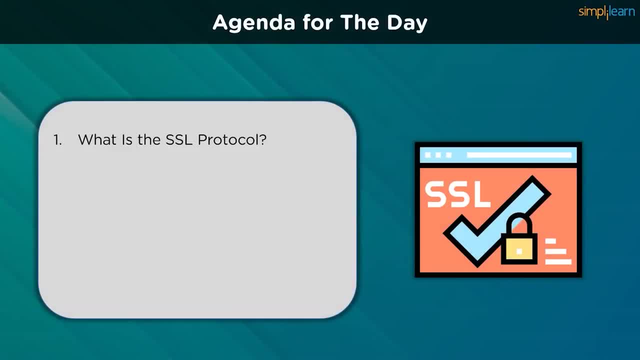 Let's look at the topics we have to cover today. We first take a look at the origin and the basics of the SSL protocol. First, let's take a look at the origin and the basics of the SSL protocol. First, let's take a look at the origin and the basics of the SSL protocol. 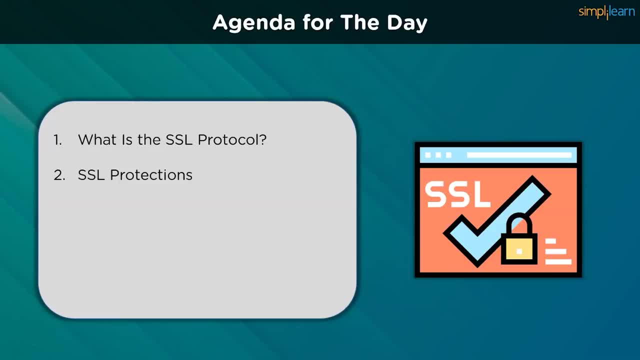 First let's take a look at the origin and the basics of the SSL protocol. UNDERHEAD, We understand the core values of the secure SSL layer and the protection it provides against various malicious attacks and domains. UN DOWN IMPLICATION: We understand the whole basis of the SSL layer and the important Turning-R poner. 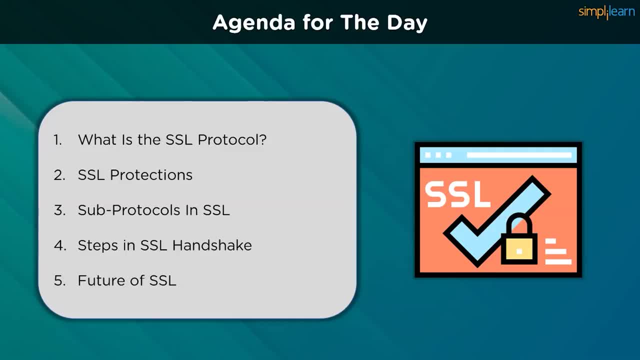 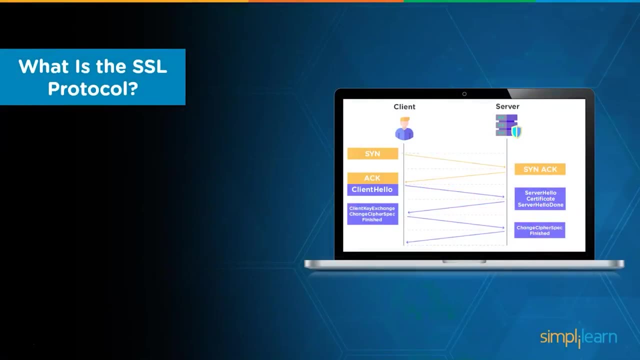 will be given in a bit CURRENT. That was H2O First. there are three factors: 1, safe supply. 2- Smart House. We also have a quiz in between the topics, so stay focused and let's see if you can answer the question. 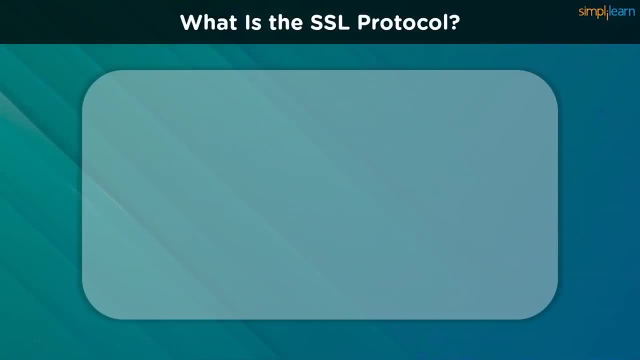 Let us learn about the SSL protocol first. SSL, or Secure Sockets Layer, is an encryption-based internet security protocol. It was first developed by Netscape in 1995 for the purpose of ensuring privacy, authentication and data integrity in internet communication. SSL is the predecessor to the modern TLS encryption used today. 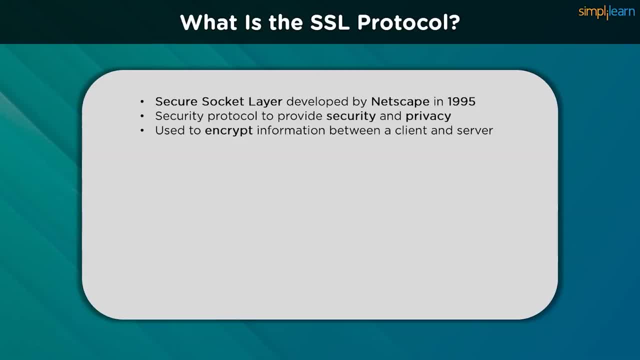 It acts as a cryptographic layer protocol that provides privacy and security to communication between a client and a web server. A website that implements SSL authentication has HTTPS in its URL instead of HTTP, In order to provide a high degree of privacy. SSL encrypts data that is transmitted across. 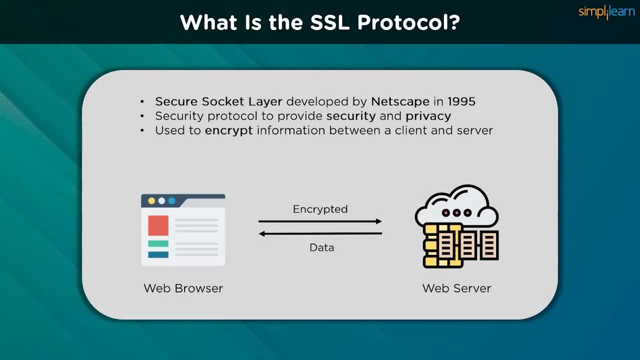 the web. This means that anyone who tries to intercept this data will only be able to access the data. SSL can only see a garbled mix of characters that is nearly impossible to decrypt. SSL initiates an authentication process called a handshake between two communicating devices. 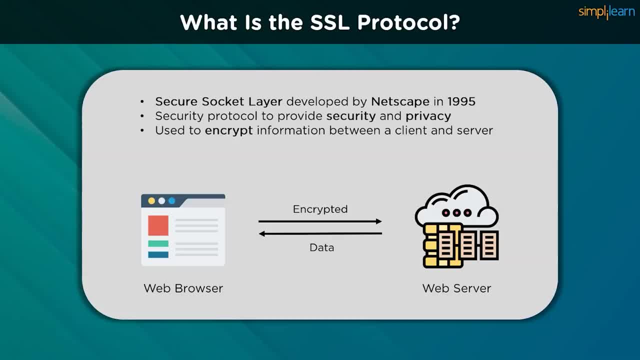 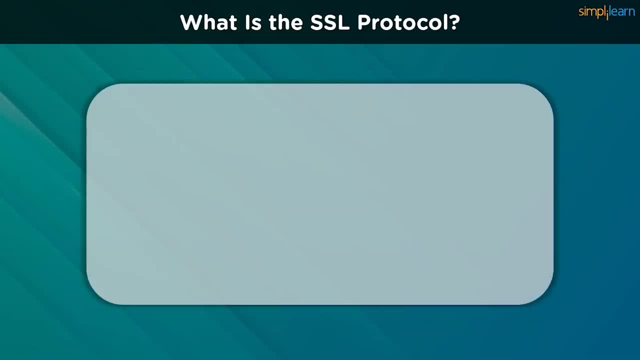 to ensure that both of them are really who they claim to be. SSL also digitally signs data in order to provide data integrity. The internet we use today follows an OSI model, or even Systems Interconnections model. It is a priority system that characterizes and standardizes the communication around. 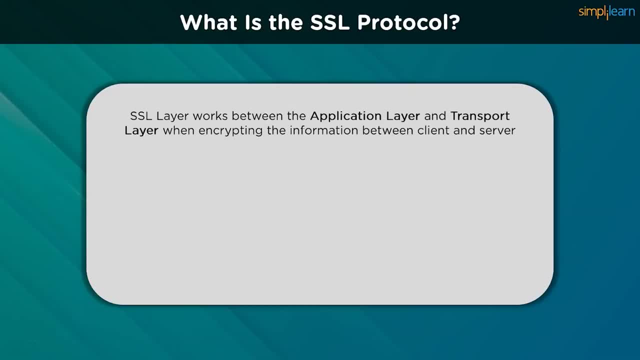 the internet Among its multiple layers. the SSL layer functions between the application layer and the transport layer. The application layer provides services for an application to ensure that effective communication with another app program is possible. The transport layer is responsible for error-free end-to-end delivery of data from the source. 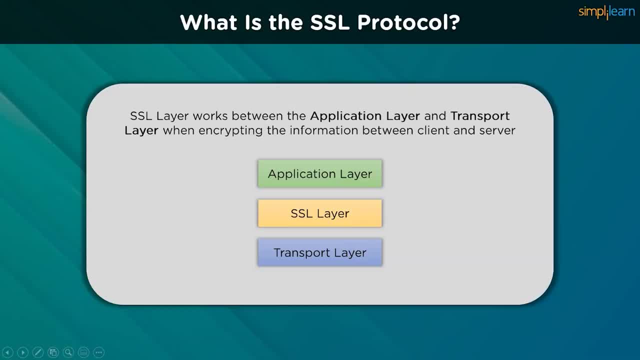 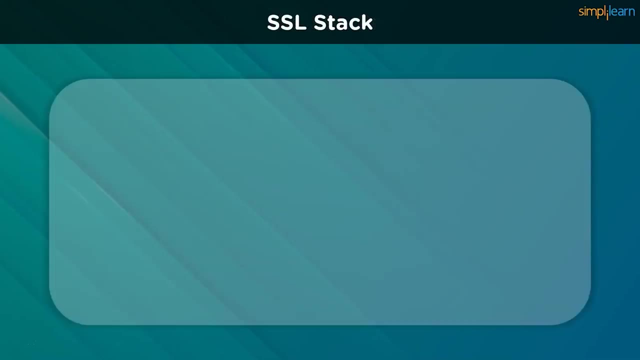 host to the destination host, Since the SSL protocol functions in between these two layers. the data is encrypted, to be encrypted, and is authenticated after being passed through the application and before it is transmitted over the network. To further understand this priority table, let us look at the table of how it works. 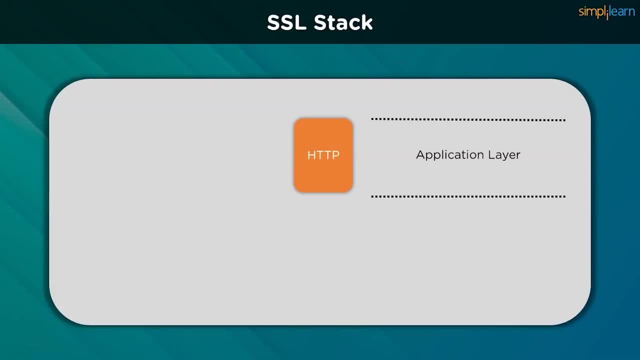 Hypertext Transfer Protocol is an application layer protocol that is used for transmitting information between computers on the World Wide Web. HTTP is based on a request-response standard between a client and server. Once the data is ready to be shared, we can pass it on to the SSL. 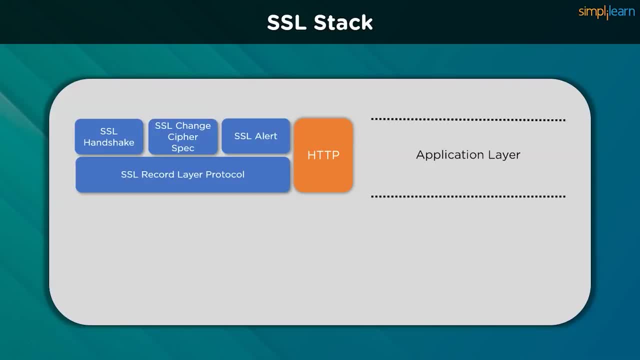 As you can notice, the protocol being used right now is HTTP. It signifies that the data is unencrypted and hence vulnerable to malicious attacks. The data is then passed on to the SSL, where we have the record protocol for the confidentiality protection and the handshake protocol for the authentication of client and server. 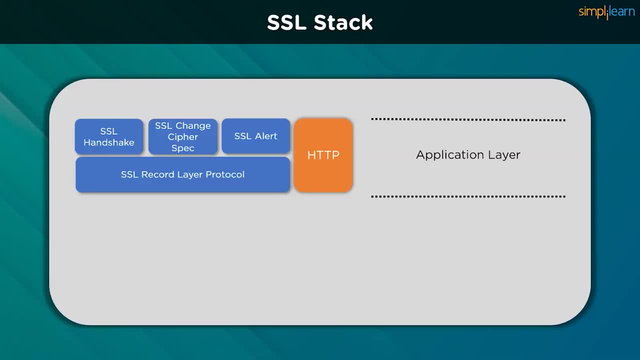 The sub-protocols of the SSL will be later discussed in detail. After the data is encrypted and ready to be transmitted, it is moved on to the transport layer, where we use the TCP packets to send that data along to the internet layer and from that point forward the data can move to its destination using the internet protocol. 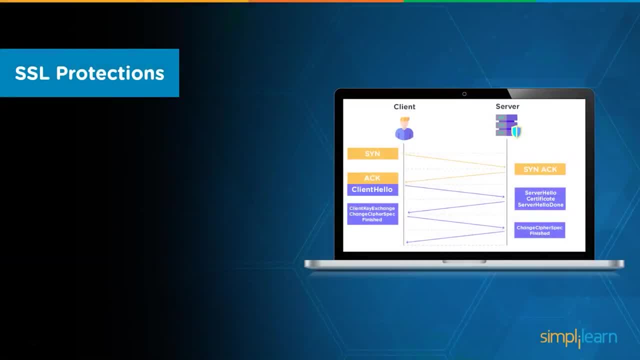 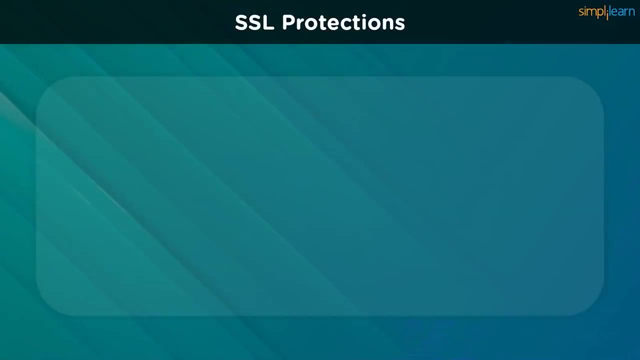 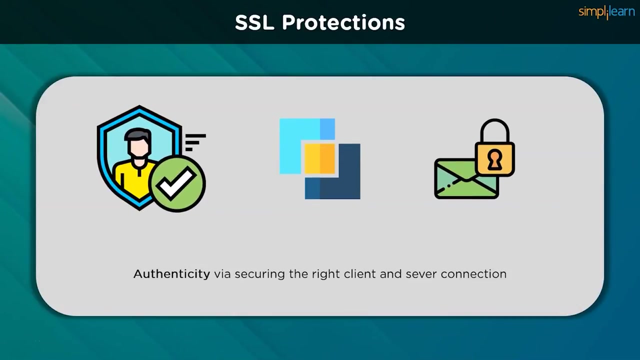 or IP addressing tables. With so many sub-protocols and sub-variants of the SSL protocol, the work is divided into multiple layers and aspects. Let's have a look at some of the ways the SSL layer make the internet safe and secure. For authentication, the client uses the server's public key to encrypt the data which is used. 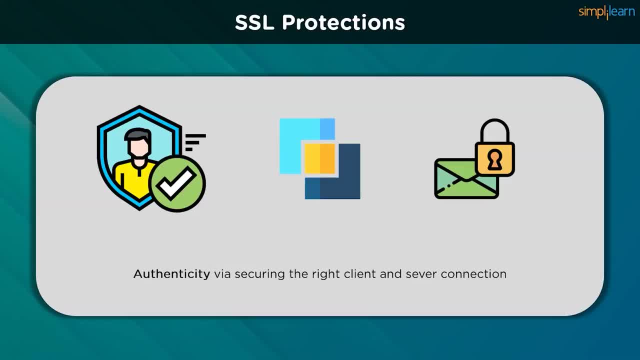 to complete the secret key. The server can generate the secret key only if it can decrypt the information with the correct private key. For client authentication, the server uses the public key in the client certificate. If any of the authentication steps fail, the handshake fails and the session terminates. 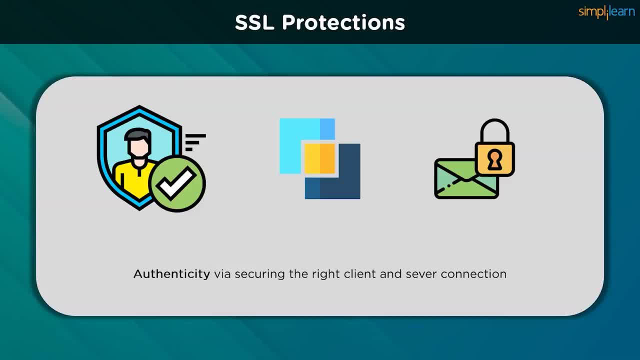 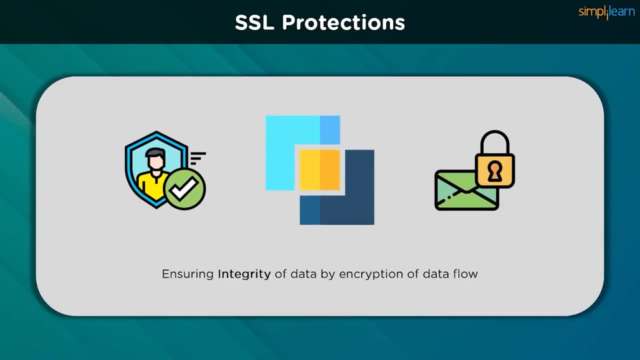 This exchange of digital certificates during the SSL handshake is a part of the authentication process. SSL provides data integrity by calculating a message digest or a hash. Use of SSL does ensure integrity, provided that the cipher spec in your channel definition uses a hash algorithm. In the SSL record protocol, the hash value is generated for the data to be transmitted. 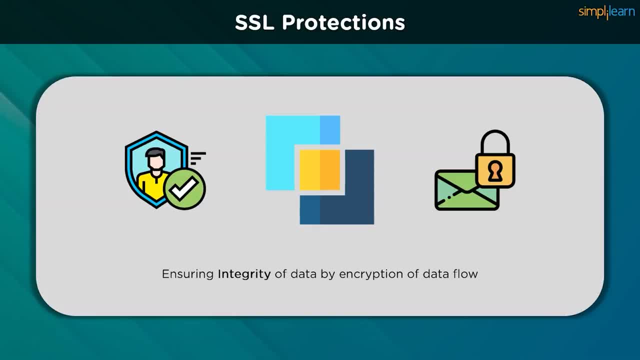 hence providing a necessary way to verify data corruption. SSL uses a combination of symmetric and asymmetric encryption. During the SSL handshake, the SSL client and server agree to an encryption algorithm and a shared secret key is used for that particular session. All the messages transmitted between the client and server are then encrypted using the same 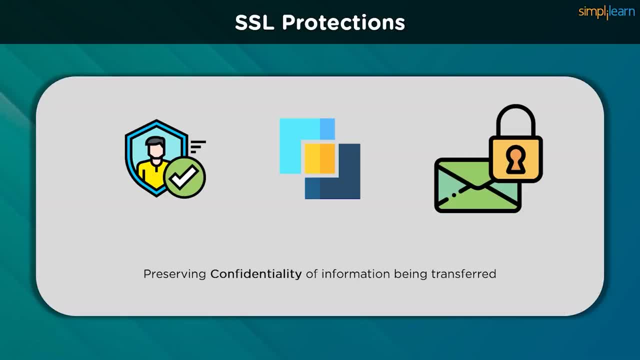 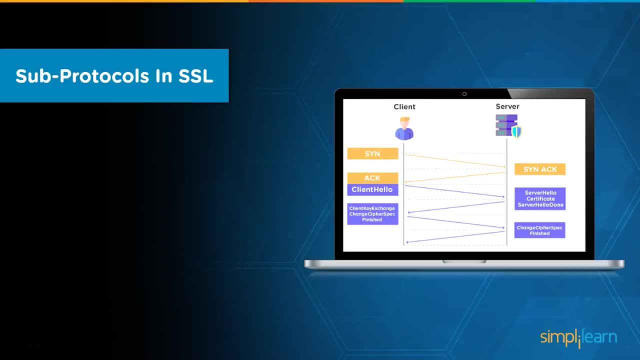 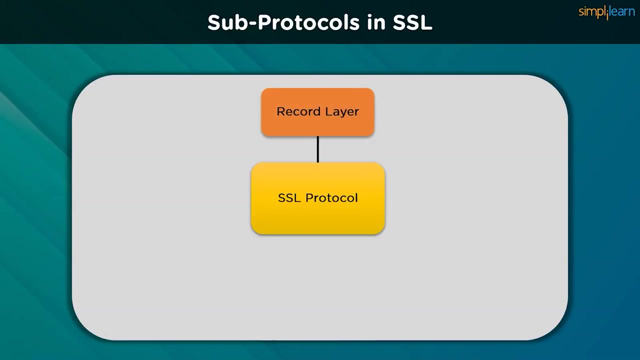 algorithm and key that ensure that the message will remain private even if it is intercepted. Regarding the multiple layers in the SSL protocol, we have many sub-protocols. The SSL record protocol provides two services to the SSL connection: confidentiality and message integrity. In SSL record protocol, the data is divided into fragments. 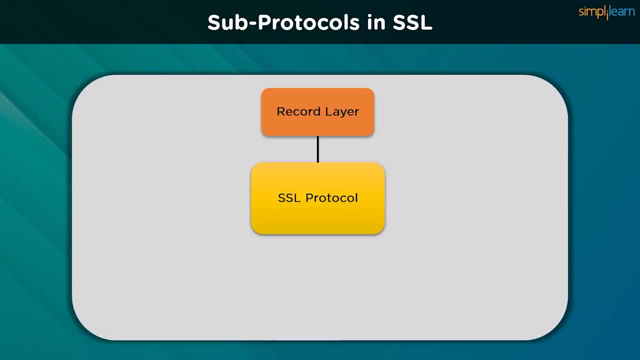 The fragment comprises of the encrypted SHA code and the MD5 code. After the encryption of the data is done, The last SSL header is also encrypted. The data is also appended to the data. The handshake protocol is used to establish sessions. This protocol allows the client and server to authenticate each other by sending a series. 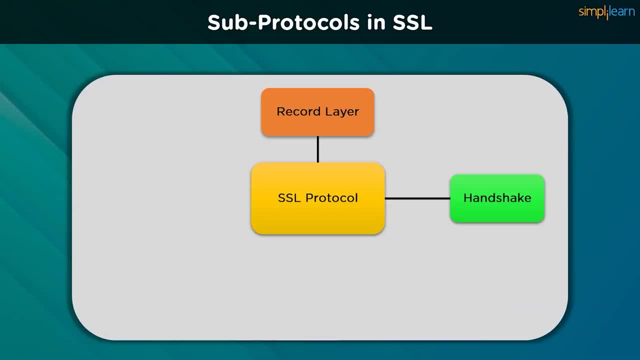 of messages. Handshake protocol uses four-phase system to complete its cycle. In phase 1, both the client and server send hello packets to each other. In phase 2, they exchange the certificates with the correct private and public keys. In phase 3, they reply to each other with a SMS. 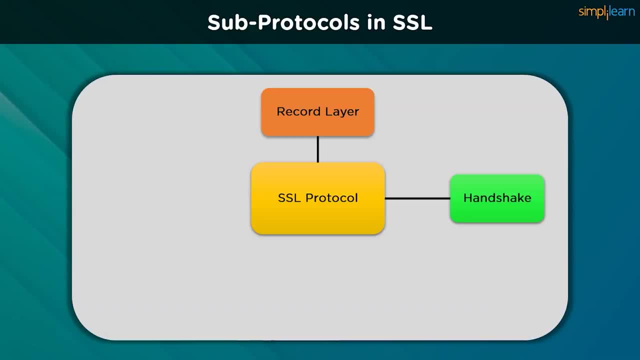 They reply to each other with the encryption algorithms and the secret keys, While in phase 4, the handshake is completed. For the chain cipher spec protocol, we use a part of the SSL record protocol. Unless handshake is completed, the SSL record output will be in a pending state. 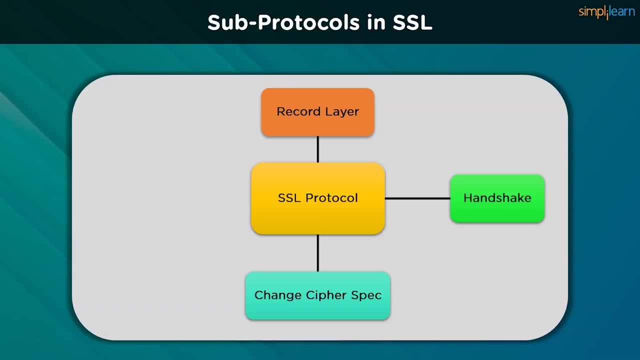 After handshake, the pending state is converted into a current state. The chain cipher protocol consists of a single message, which is of one byte in length and can hold only one message. The SSL alert protocol is used to convey SSL-related alerts to the peer entity. 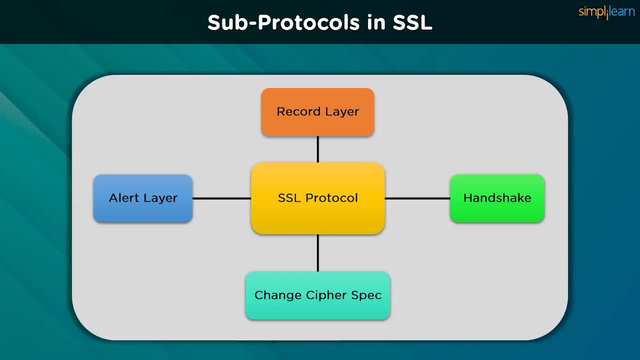 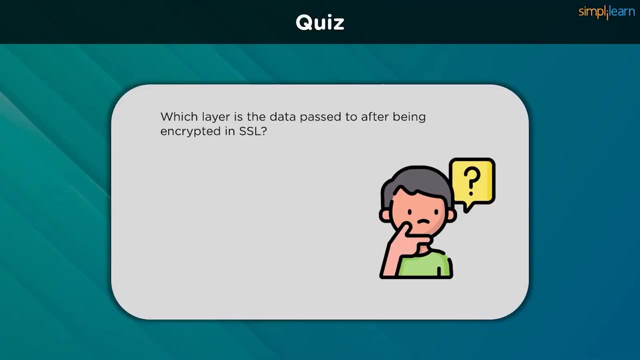 Each message in this protocol contains only two bytes. Let's take a small quiz to check if the older topics are clearly understood. Once the data is encrypted in the SSL layer, where is the data being passed on to? Is it A? The application layer? B- The transport layer? 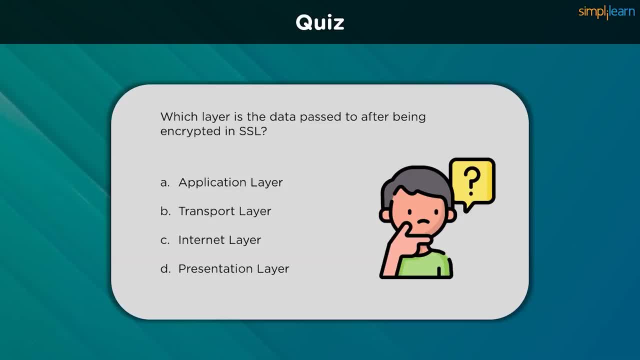 C- The internet layer, Or D- Presentation layer. Take a few seconds to recall our last topic and be sure to leave your answer in the comments section of this video. Let's move on with our topic. Now that we understand the entire protocol and its working, let's see how the SSL handshake. 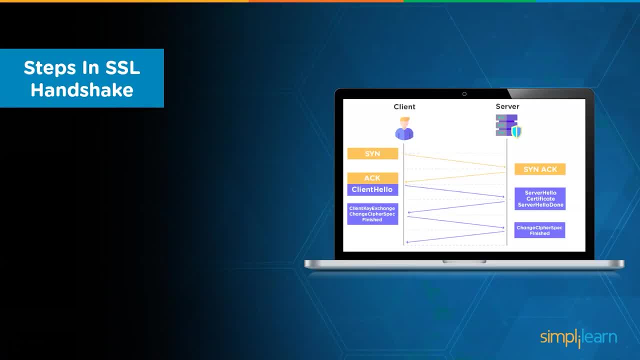 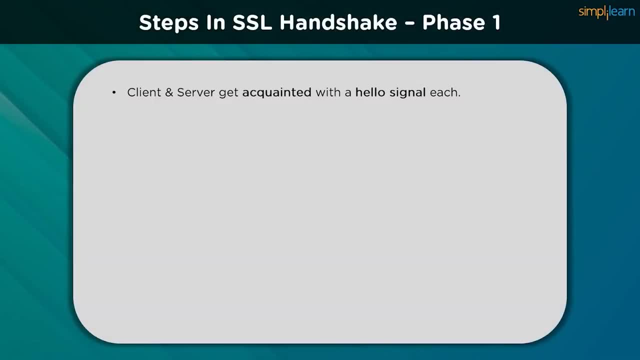 works in a step-by-step format. We have divided the handshake into four distinct phases. In phase 1, the client and server get acquainted with the hello signal message from each side. The client sends the SSL version. In phase 2, the server sends the SSL version of the SSL to the client and the SSL returns. 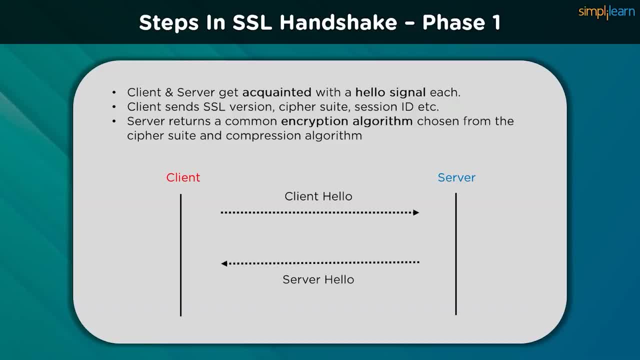 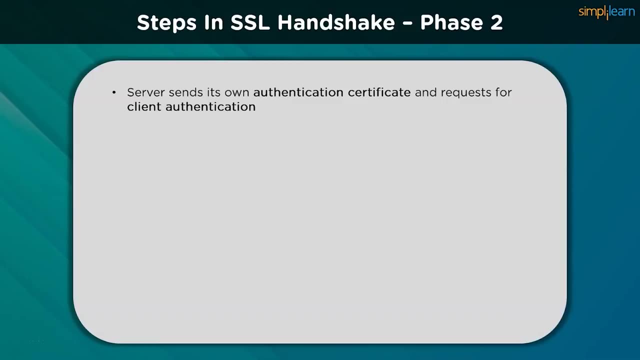 an encryption algorithm which is chosen from the cipher suite and a compression algorithm which is sent from the client hello signal each. This helps in setting up a common encryption algorithm and a common hash value to be used throughout the handshake process. In phase 2, the server sends its authentication certificate and requests for client authentication. 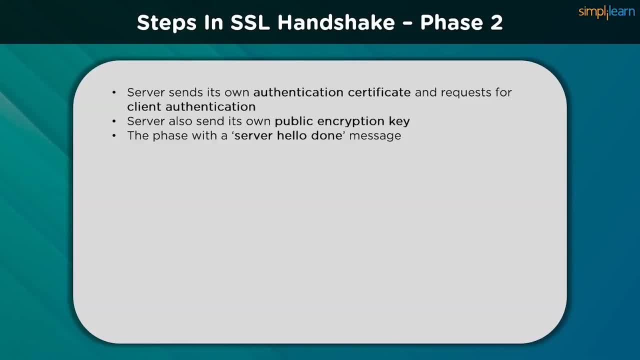 The server sends its public encryption key and the phrase with the server- hello done. message. Once the server sends its public key, the client can use it to encrypt its own private key, which will be later used to encrypt the data being exchanged between the client and. 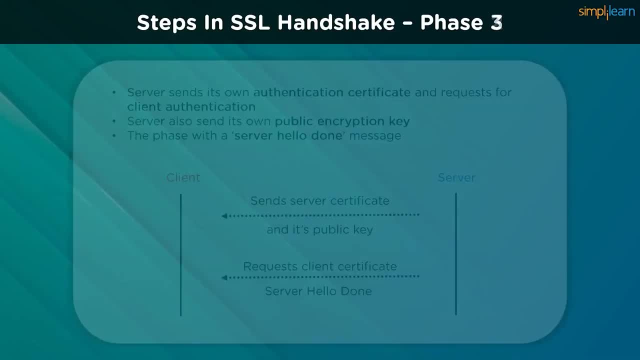 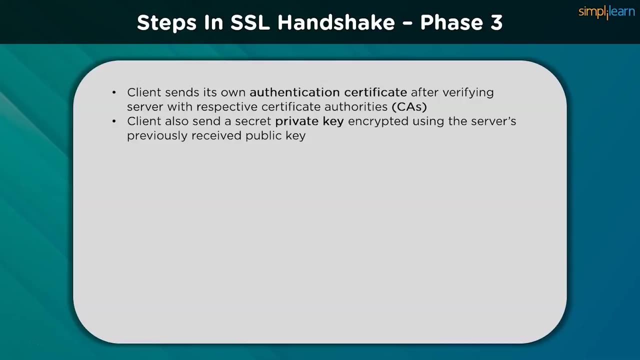 a server. In phase 3, the client sends its authentication certificate after verifying the server with the respective certificate authorities. There, the client now sends the public key- private key- which is encrypted using the server's previously sent public key. In phase 4, the client sends the status of the cipher functions, along with a finished 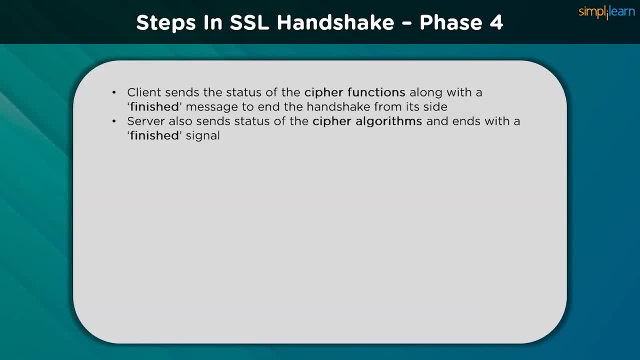 message to end the handshake. from its side, The server also sends the status of the cipher algorithm and ends with a finished signal. The data is now encrypted with the symmetric key client sent in phase 3.. With the end of phase 4, authentication is complete and the SSL handshake has maintained. 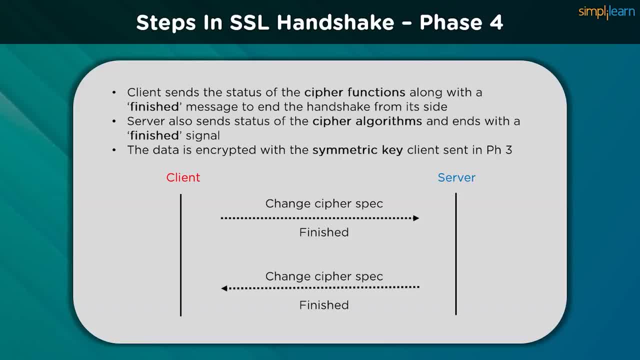 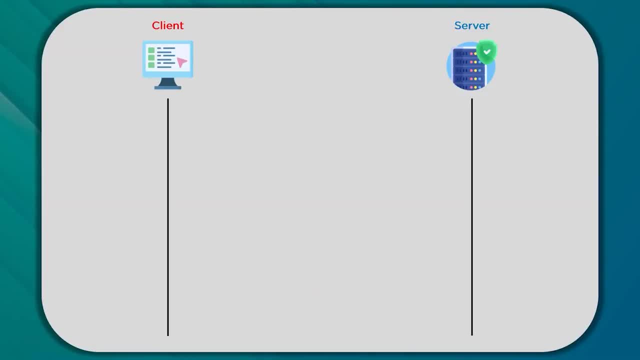 the authenticity of the entire session between the client and server. To reiterate the entire process, let's go through each step one more time. The client sends a hello request to the server, The server responds with its own hello message and sends the server authentication certificate. 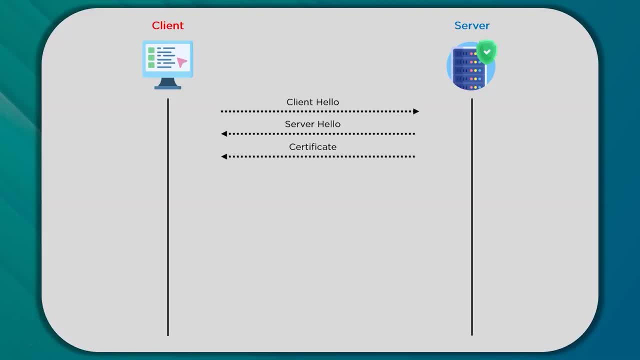 for verification. At this point the server's hello signal is complete. The client exchanges a secret key with the server to encrypt the data and the cipher spec parameters are changed accordingly. The client has now finished its own handshake activities. The server uses the secret key provided by the client to encrypt the data and alters. 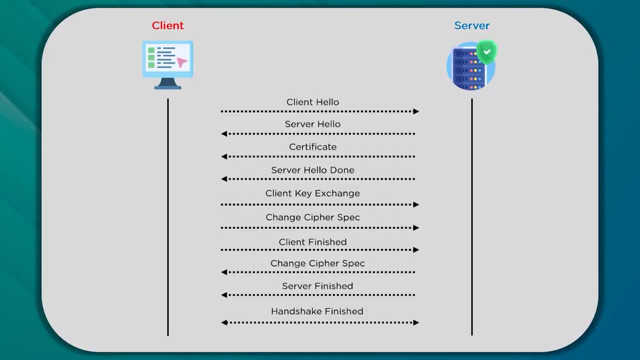 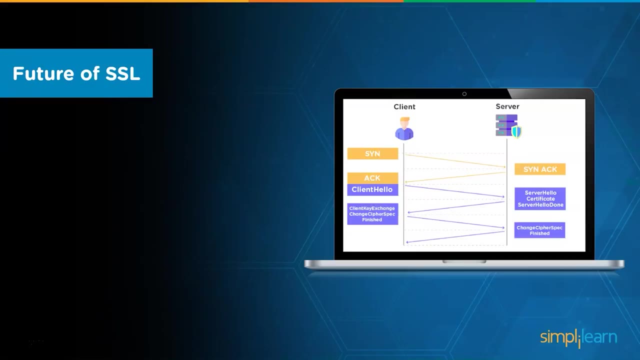 its own cipher spec parameters as a final step before it sends a finished signal. At this point, the SSL handshake is complete, with an encryption algorithm and a secured data channel. With the SSL protocol being developed in the early 90s, it was bound to be a little. 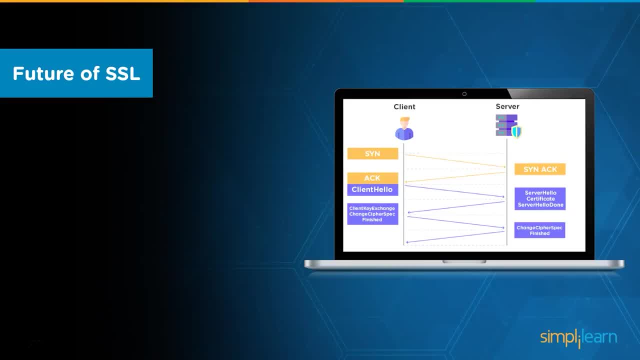 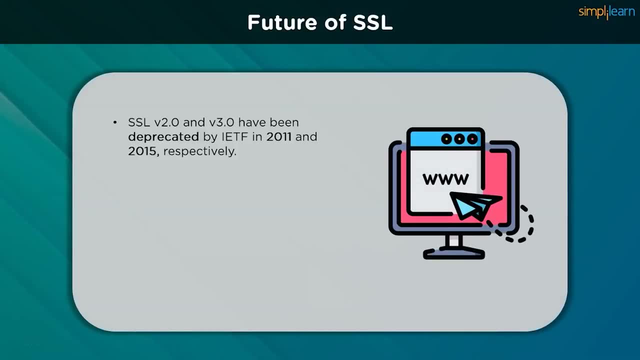 underpowered when pitted against the current day computers and hackers. Let's see its future implications and replacements. SSL encryption has been depreciated now, with its version 2 and version 3 being dropped by the Internet Engineering Task Force in 2011 and 2015 respectively. 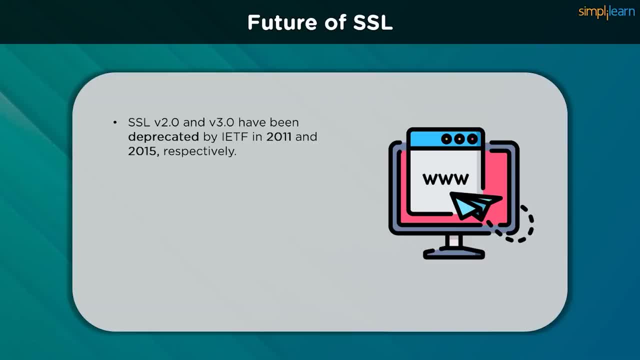 There are different ways to encrypt SSL encryption. For example, if you want to encrypt SSL encryption, you need to use the Internet Engineering Task Force. There have been far too many security vulnerabilities to carry on official activities during the SSL era. To further enhance the security, the Transport Layer Security, or TLS, has been developed. 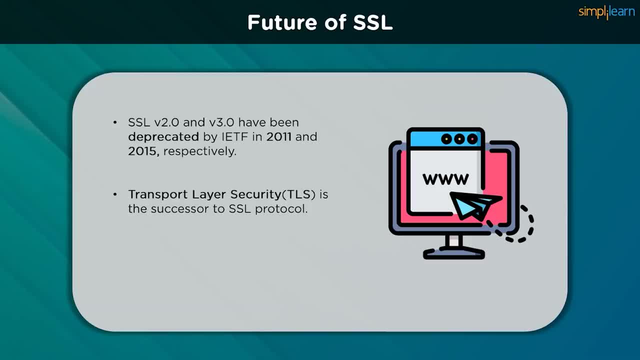 as a successor to the SSL protocol. TLS is a proposed IETF standard first developed in 1999, and the current version is TLS 1.3, which was defined in August 2018.. Even though a major part of the Internet is still using TLS 1.2 as a safety net, the transition